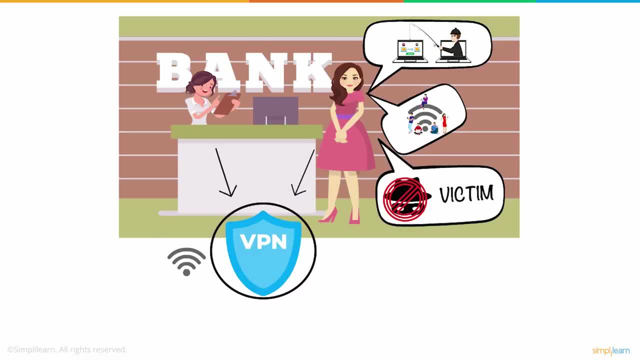 Like most of us, Jude had come across the term VPN several times but didn't know much about it. She was very concerned about the security of her bank account, She was worried that her bank wallet, and little did she think that the repercussions of not using a VPN would be this. 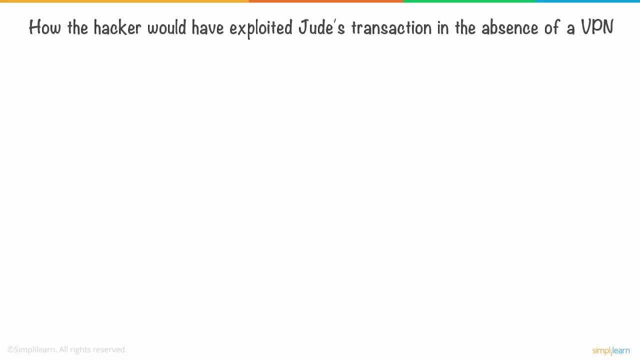 bad. Let's understand how the hacker would have exploited Jude's transaction in the absence of a VPN. In this process, Jude's computer first connects to the internet service provider, ISP, which provides access to the internet. She sends her details to the bank's server using her IP. 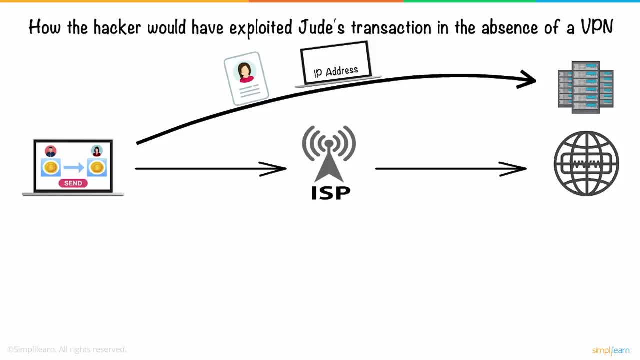 address, Internet protocol address or IP address is a unique address that recognizes a particular device. The IP address is a unique address that recognizes a particular device. The IP address is a unique address that recognizes a particular device, be it a laptop or a smartphone on the. 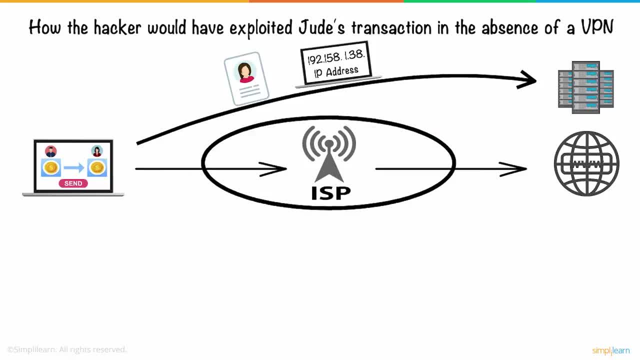 internet. When these details pass through the public network, the hacker, who passively watches the network traffic, intercepts it. This is a passive cyber attack where the hacker collects Jude's bank details without being detected. More often or not in such an attack, payment information is likely to be stolen. The targeted data here are the victim's username. 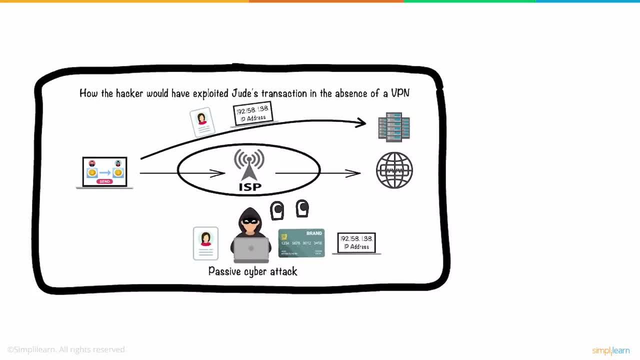 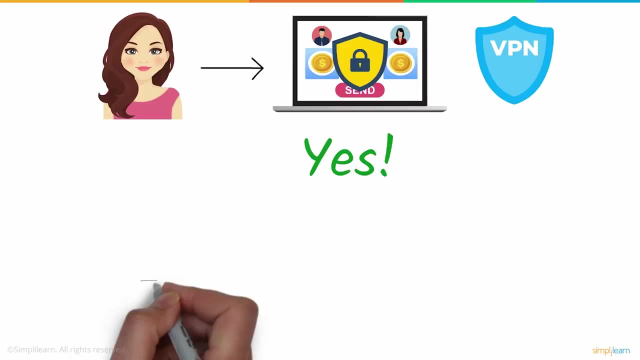 passwords and other personal information. Such an unsecured connection exposed Jude's IP address and bank details to the hacker when it passed through the public network. So would Jude have been able to secure her transaction with the help of a VPN? Well, yes. Picture Jude's bank transaction to be happening in a tunnel that is invisible to the 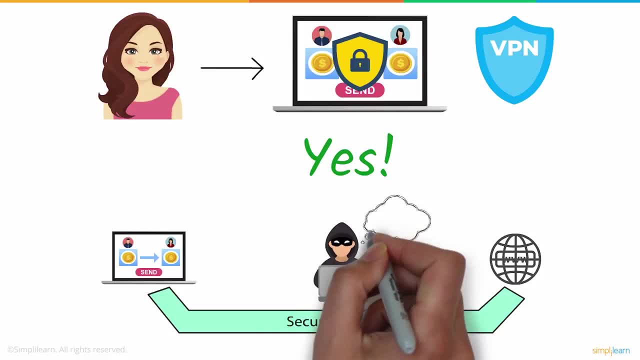 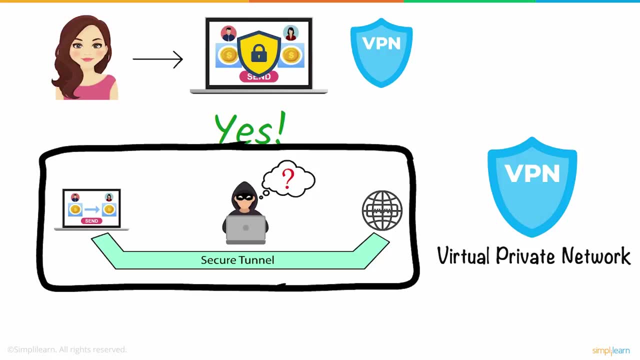 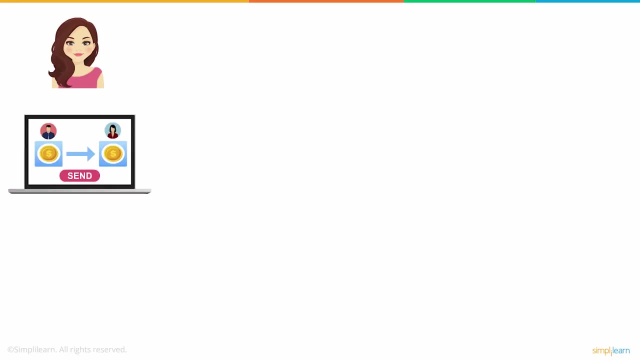 hacker. In such a case, the hacker will not be able to spot her transaction, and that is precisely what a VPN does. A virtual private network, more often known as VPN, creates a secure tunnel between your network and the internet. For using a VPN, Jude's first step would be to install software-based 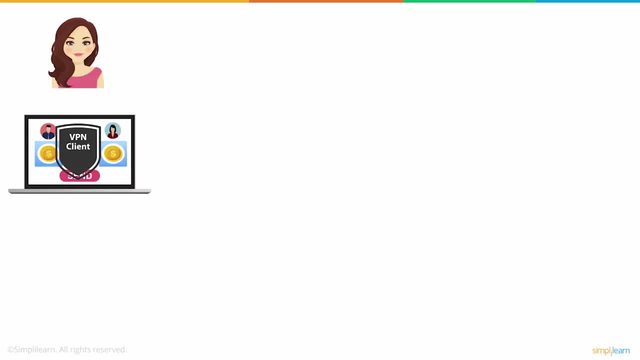 technology, known as the VPN client, on her laptop or smartphone. that would let her establish a secure connection. The VPN client connects to the Wi-Fi and then to the ISP. Here the VPN client encrypts Jude's information using VPN protocols. Data is encrypted to make sure it is secure. 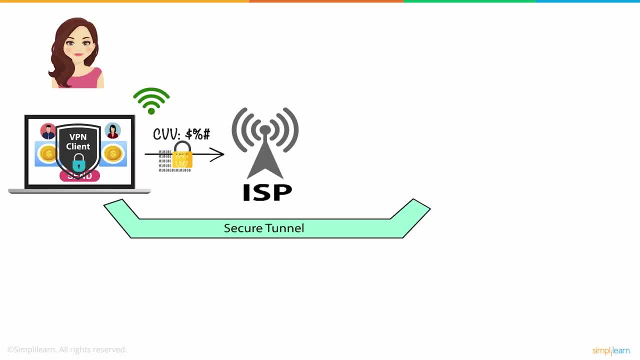 Next, the VPN client establishes a VPN tunnel within the public network that connects to the VPN server. The VPN tunnel protects Jude's information from being intercepted by the hacker. Jude's IP address and actual location are changed at the VPN server to enable a private and secure connection. Finally, the VPN server connects to Jude's bank. 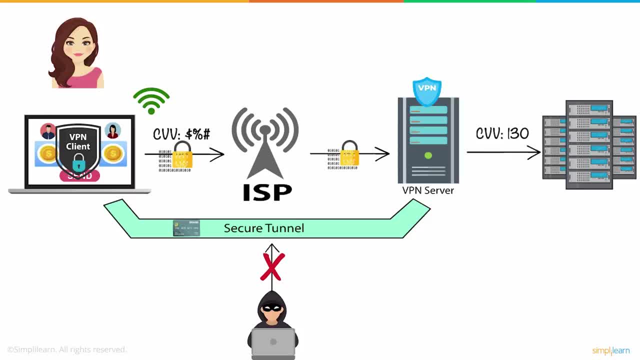 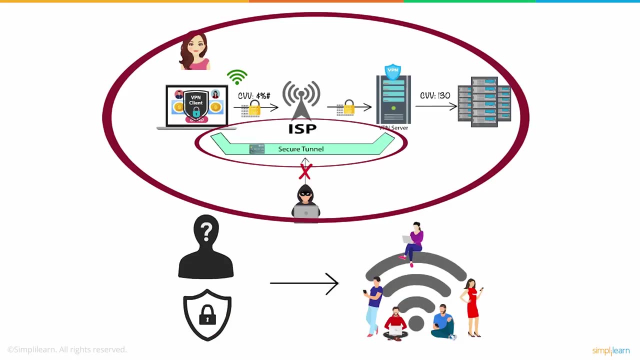 server in the last step, Where the encrypted message is decrypted. This way, Jude's original IP address is hidden by the VPN, and the VPN tunnel protects her data from being hacked. how VPN makes your data anonymous and secure when it passes through the public network. 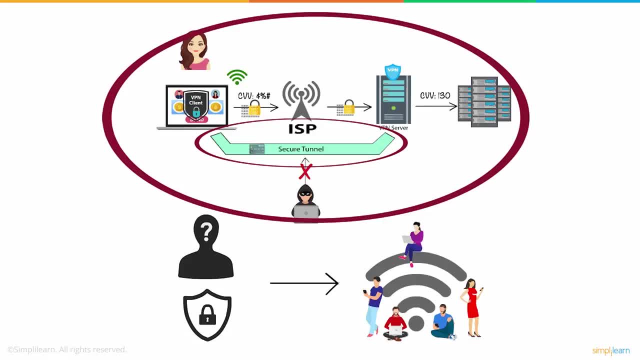 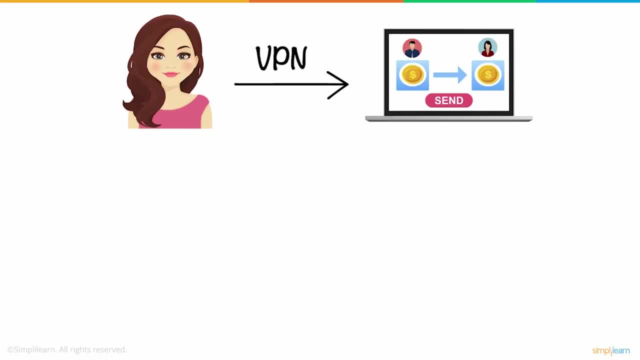 and the difference between a normal connection and a VPN connection. After learning about this, Jude was certain that she should start using a VPN to carry out her online transactions in the future. This is also applicable to each one of us, Even if you work remotely or connect to public Wi-Fi. 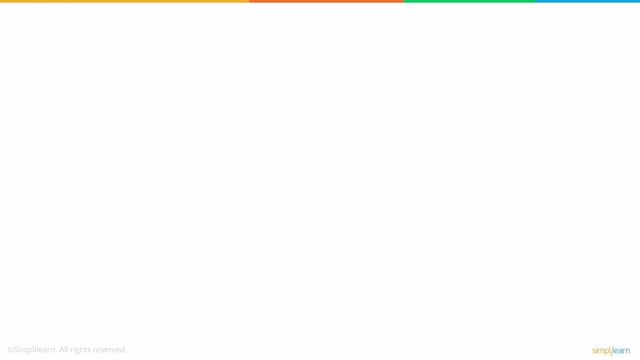 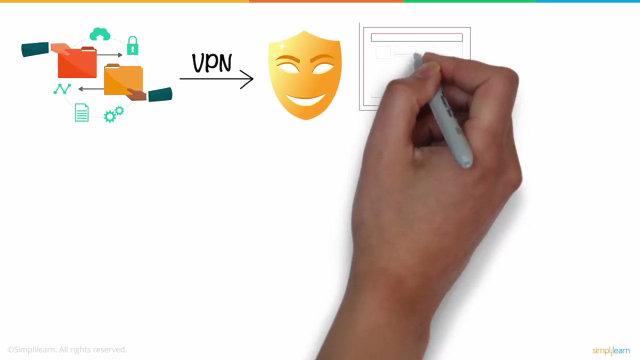 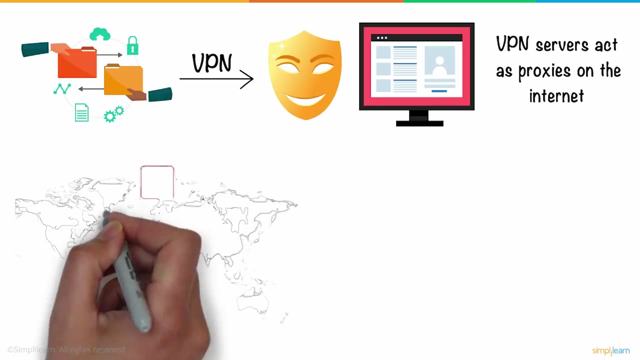 using a VPN is the safest option. In addition to providing a secure, encrypted data transfer, VPNs are also used to disguise your whereabouts and give you access to regional web content. VPN servers act as proxies on the internet. This way, your actual location cannot be established. 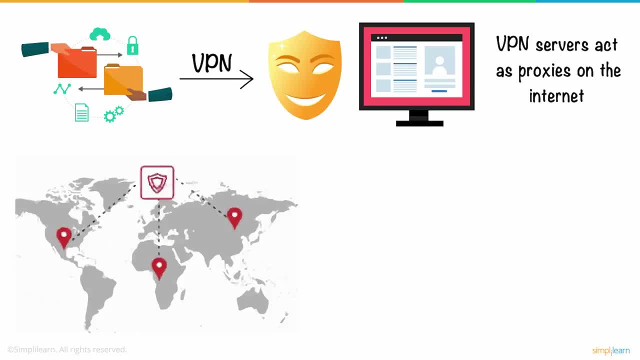 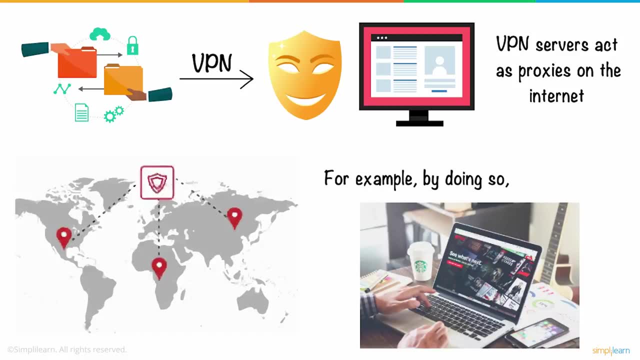 VPN enables you to spoof your location and switch to a server to another country and thereby change your location. For example, by doing so, you can watch any content on Netflix that might be unavailable for your region. So here's a question for you. 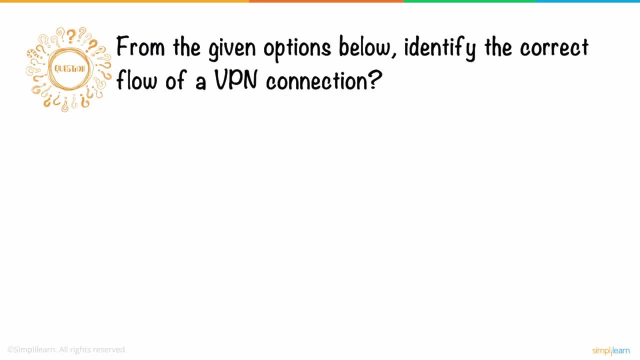 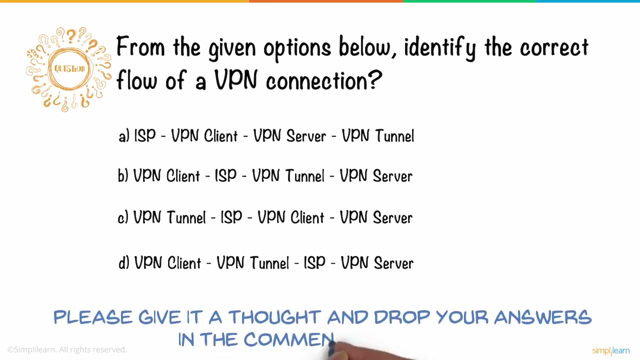 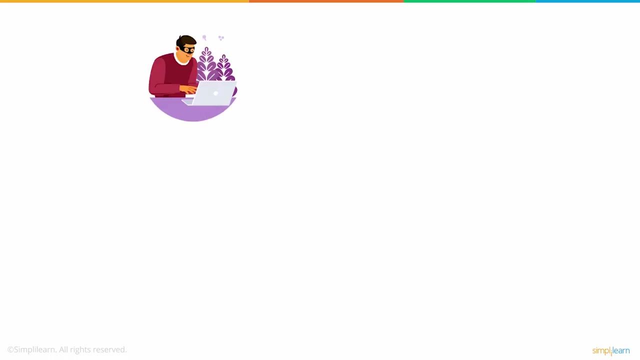 From the given options, identify the correct flow of a VPN connection. A, B, C, D. Do give it a thought and leave your answers in the comments section below. Three lucky winners will receive Amazon gift vouchers. Given the current scenario, 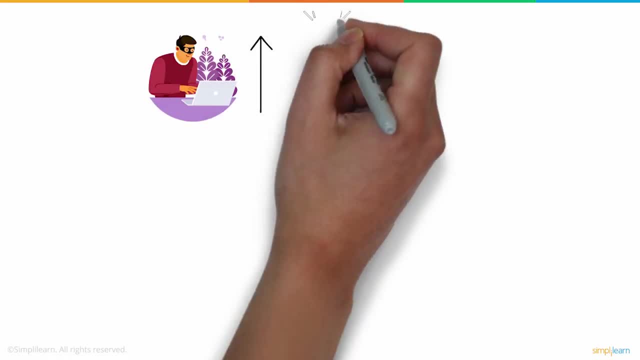 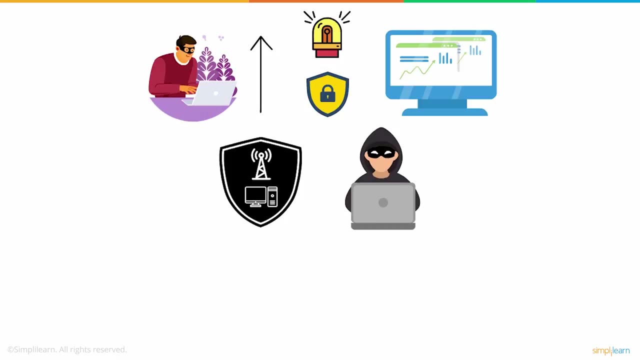 cyber attacks are on the rise now more than ever, So we have to stay alert and protect our digital information. If you are interested in protecting networks and computers from cyber criminals, a cybersecurity career is what you should venture into. So what are you waiting for?